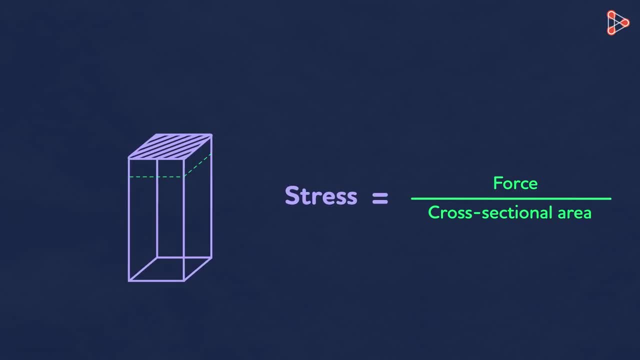 Mathematically stress is defined as force per unit cross-sectional area. So it is F over A. where A is this cross-sectional area? What if I increase the force from F newton to say F plus 10 newton on this area A? 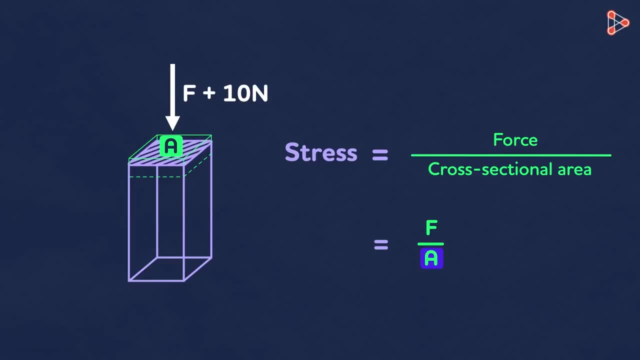 Intuitively we know that if we push it with a greater force from above, then the beam will experience more stress. Mathematically, this new stress will be F plus 10 over A. The numerator increased and the denominator remained the same. It means that the beam will experience more stress. So it is F over A, where A is this cross-sectional area. Mathematically, this new stress will be F plus 10 over A. It means that this ratio is greater than this one. 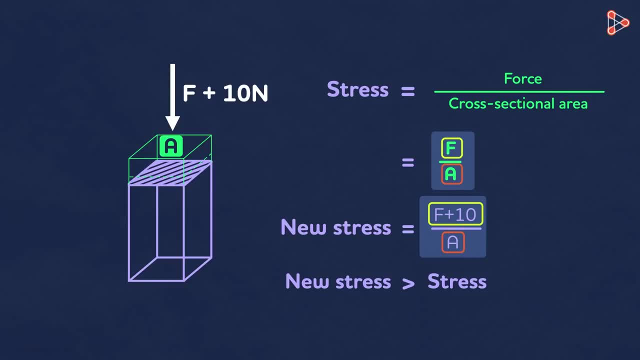 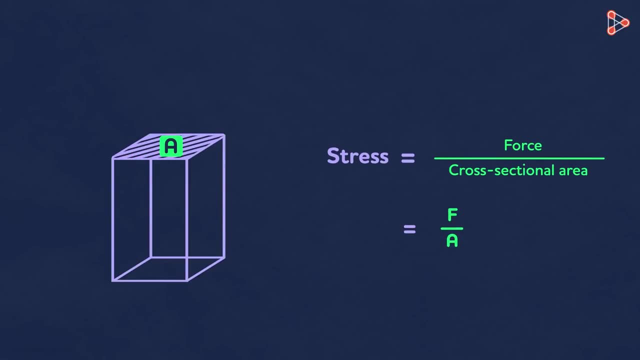 So if we increase the force, the stress will also increase. Next, what will happen if I increase the surface area from A meter squared to say A plus 10 meter squared? Will the stress increase in this case too? The stress will decrease in this case because the denominator increases with the numerator remaining constant. 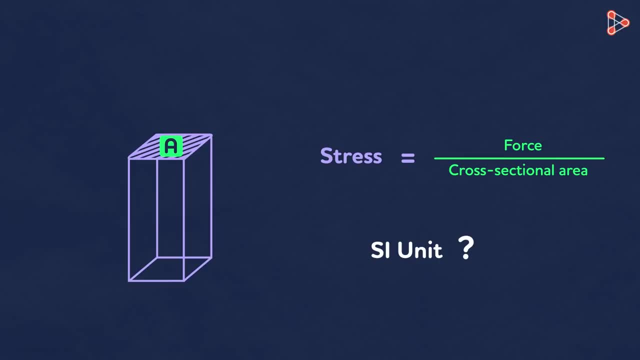 Now, what is the SI unit of stress? Any guesses? Stress is force per unit area. The SI unit of force is newton, denoted by n, and that of area is meter squared. So the SI unit of stress is newton per meter squared. 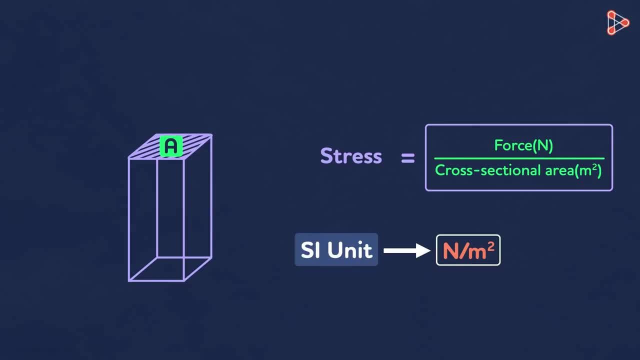 However, this unit is given a name and it is called Pascal, denoted by PA. Now we know the basics about stress. What is strain? In very simple language, one can define it as change in dimensions per unit of original dimensions. When any object is under stress, it will change one or more of its dimensions. 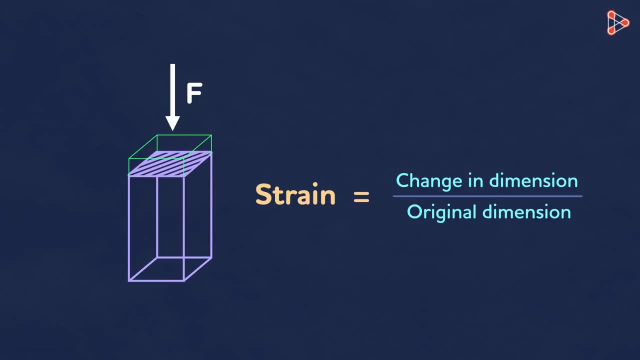 The amount by which the object's dimensions will change will depend on the force applied and the materials the object is made up of. In our example, L is the length of the beam and it's experiencing some force, Hence it will deform and its length will be the same. 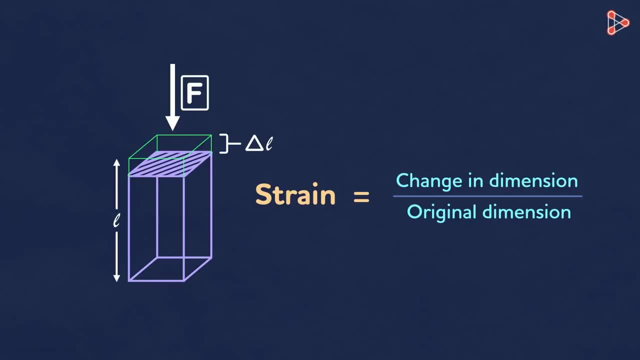 Hence its length will change by, say, delta-L Strain is defined as change in length per unit of the original length. Mathematically, it is delta-L over L. So what does this ratio do? Well, the ratio compares the change in length that resulted due to force with the original length of the beam.